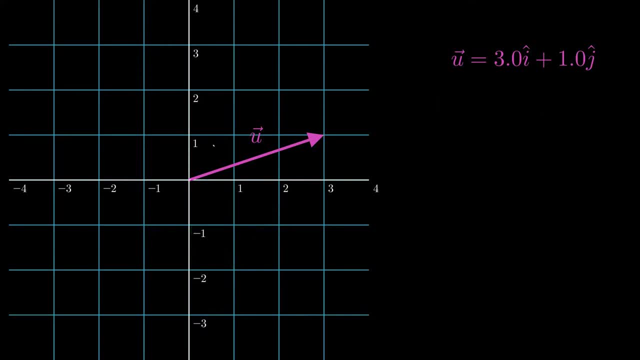 Same result, both methods. Next we're going to be looking at the unit vector. Next we're going to be exploring the unit vector. The unit vector is a vector in the same direction as a given vector, but it only has a magnitude of 1.. 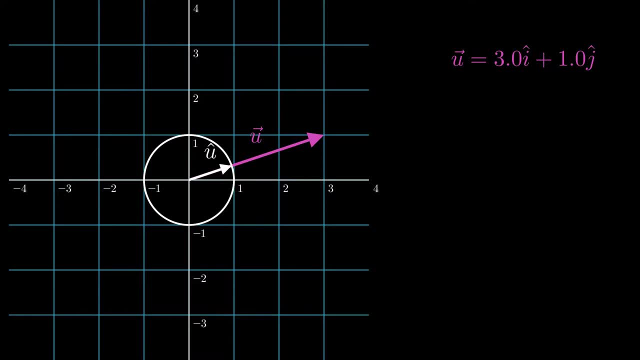 I've drawn a unit circle to emphasize that point. The white vector will always be touching the unit circle. The equation for the unit vector is the given vector divided by its magnitude. In this case it's 3 i-hat plus 1 j-hat over the square root of 3 squared plus 1 squared. 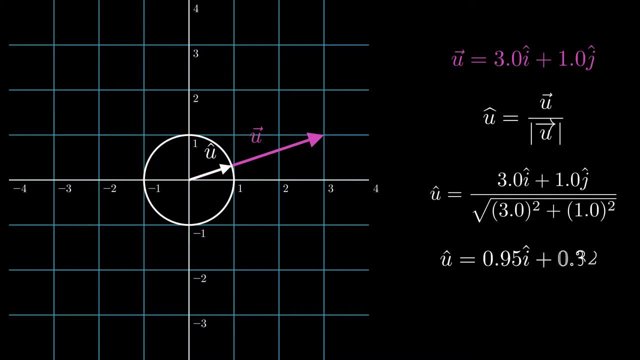 Similar to Pythagorean Theorem, The result is 0.95 i-hat plus 0.32 j-hat. If we're to shift the pink vector to the left, you'll notice that the pink vector's length is shrinking, while the white vector's is staying the exact same length, but it's changing because it's following the pink direction. 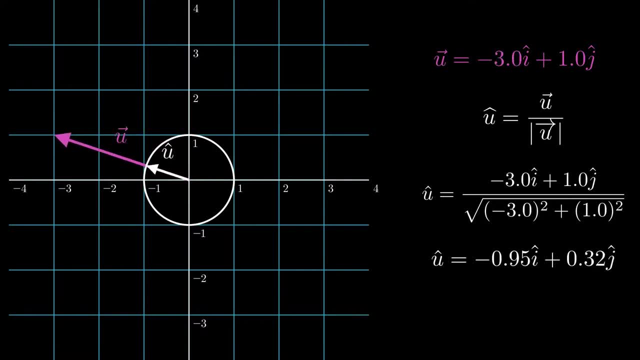 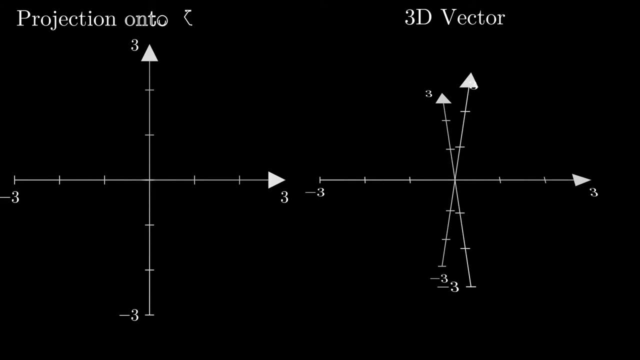 That's an example of the unit vector always staying at magnitude 1.. Now it's time to move on to the Calculus 3, part 3 dimensions. On the right you have our 3D view. On the left you have a top-down approach of that 3D view. 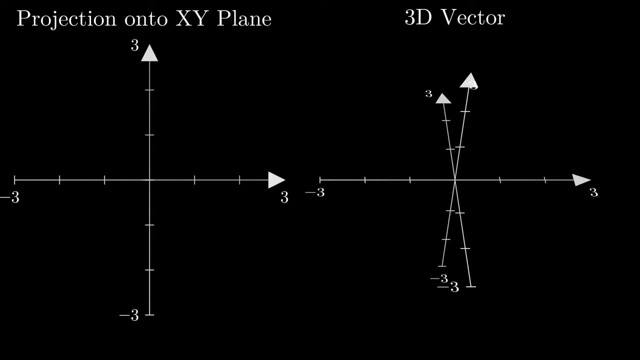 So we're looking directly from above it. Left is the xy-plane. If we draw the same vector on both sides, this is another vector called u. this is what it would look like: The right is the 3D, the left is directly looking down on top of it. 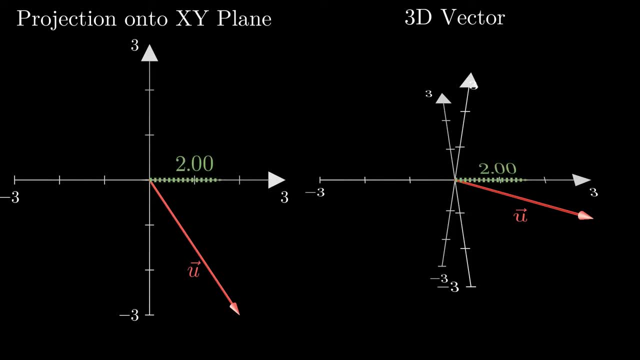 This vector has 2 in the x-direction, negative 3 in the y-direction and positive 2 in the z-direction. You'll notice on the left that you don't see any yellow line because you're looking directly down on top of it. 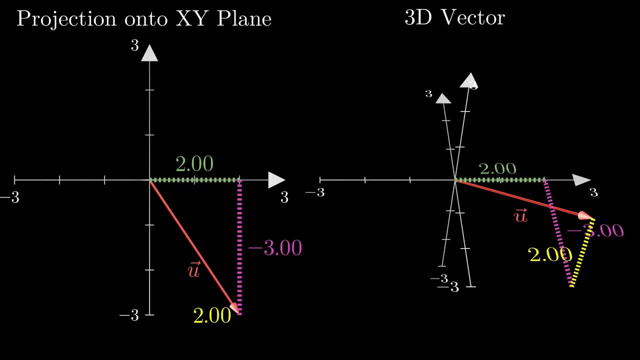 We're going to look at the unit vector again. I've drawn a sphere of radius 1 on the screen. On the left it looks like a circle because it's top-down view. We're just viewing the cross-section. On the right, it looks like a sphere because that's what it is.